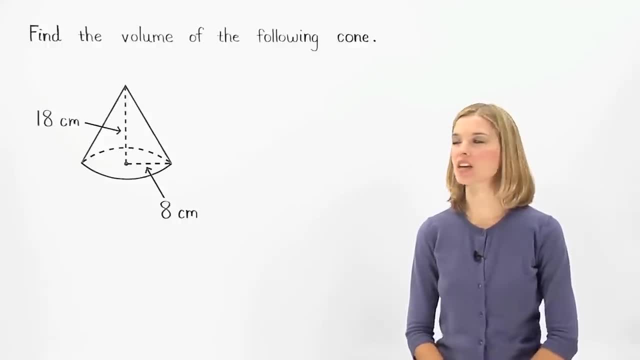 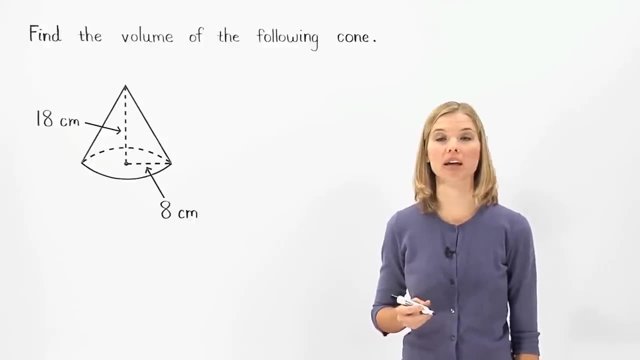 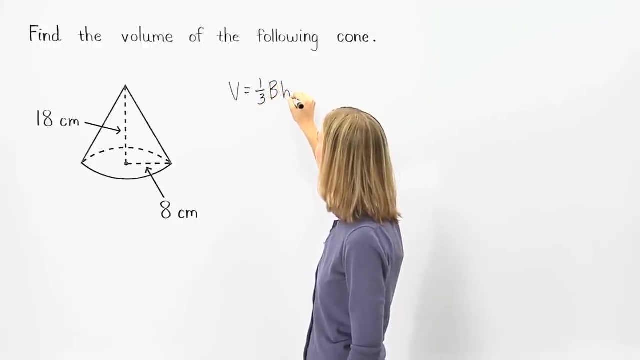 In this example, we're asked to find the volume of the given cone. To find the volume of a cone, we use the same formula that we use to find the volume of a pyramid. Volume equals one-third times area of the base times height. 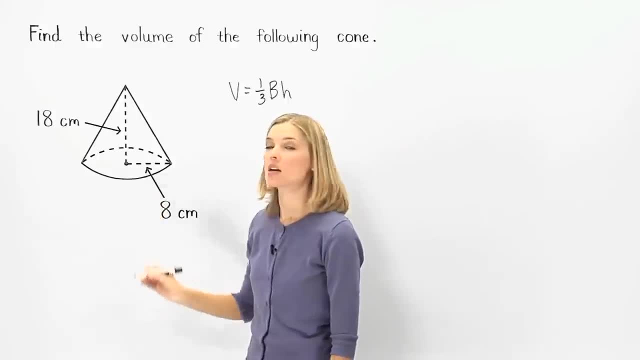 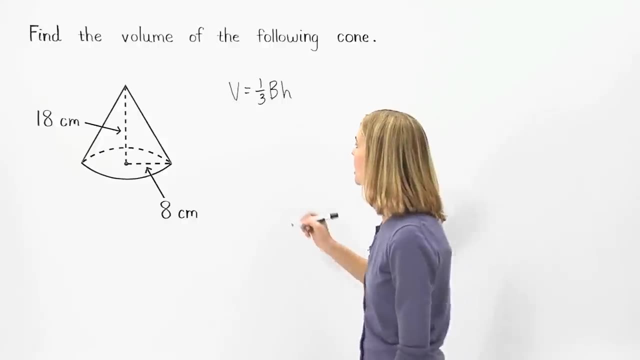 Notice, however, that the base of a cone is a circle And remember that the formula for the area of a circle is pi times radius squared. So another way to write the formula for the volume of a cone is: volume equals one-third times pi times radius squared times height. 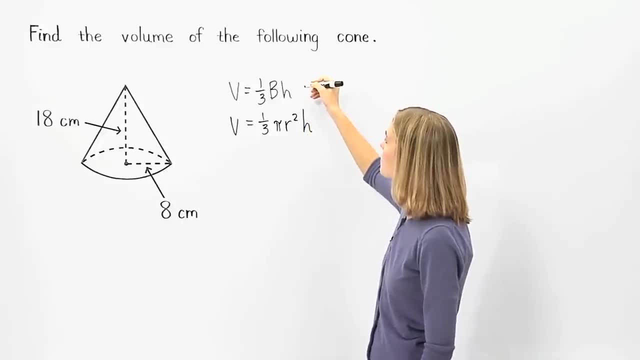 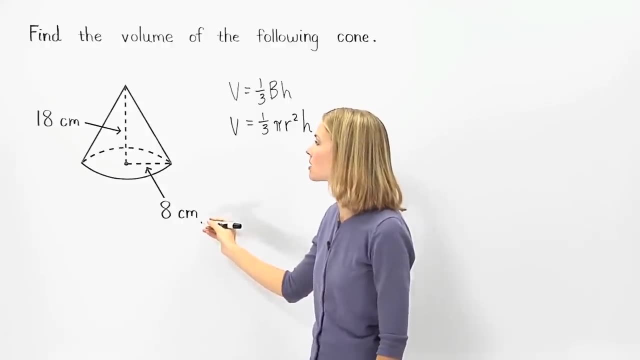 which is the same thing as one-third times area of the base times height. So to find the volume of the given cone, since the radius is 8 centimeters and the height is 18 centimeters, we can plug this information into the formula to get. 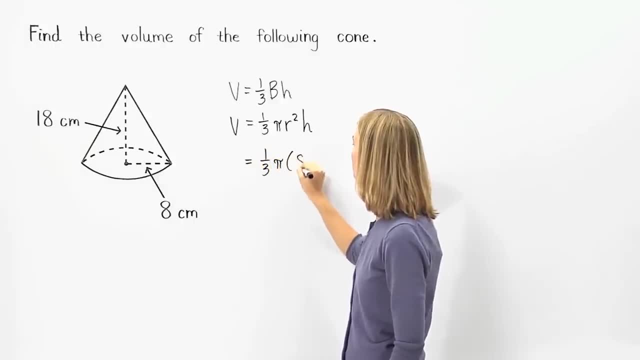 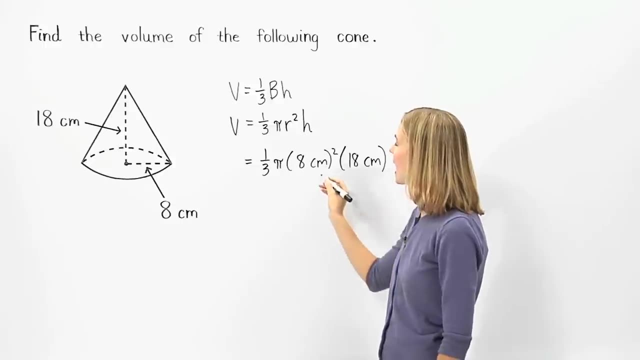 one-third pi times 8 centimeters squared, times 18 centimeters. Remember that 8 centimeters squared is the same thing as 8 centimeters times 8 centimeters, which equals 64 centimeters squared, And we have one-third pi. 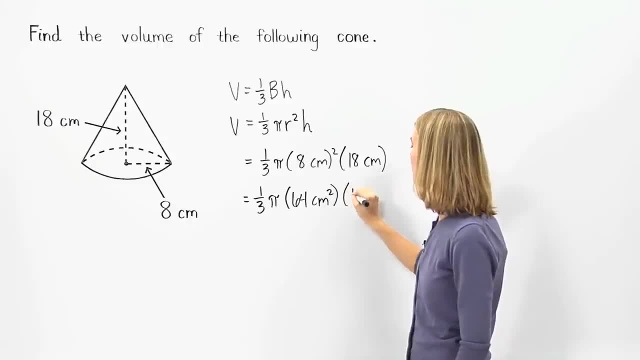 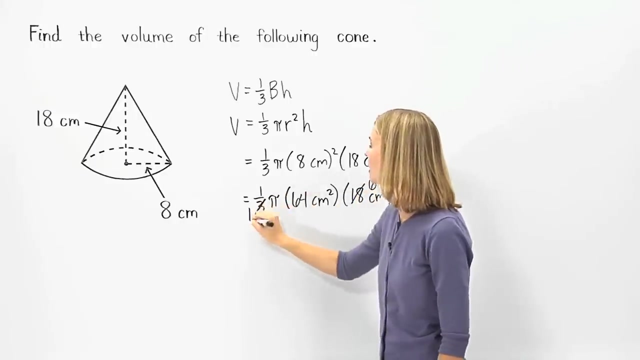 times 64 centimeters squared, times 18 centimeters. Simplifying from here, I would multiply one-third times 18. next, Notice that 18 and 3 cross-cancel to 6 and 1.. And we have one times pi times 64 centimeters squared. 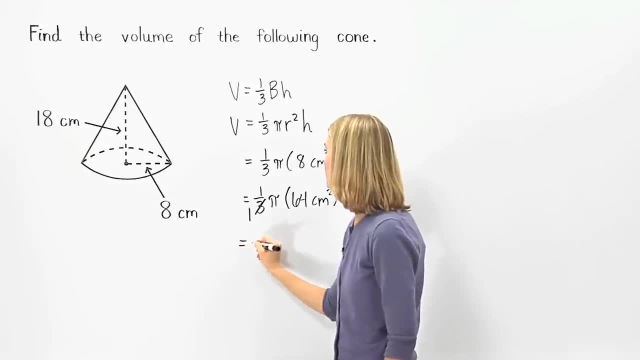 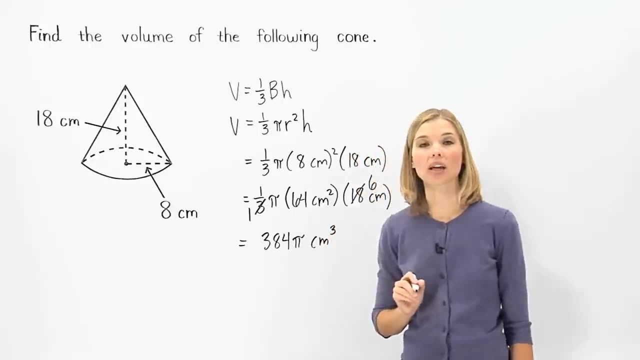 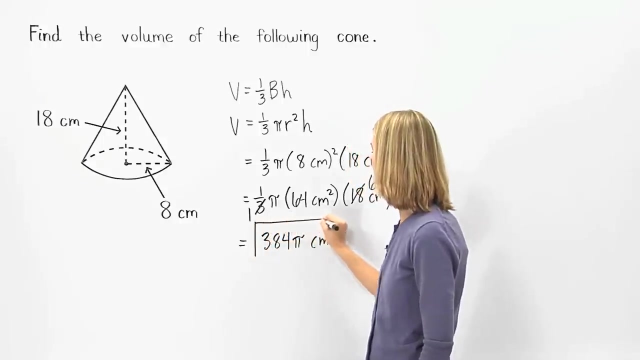 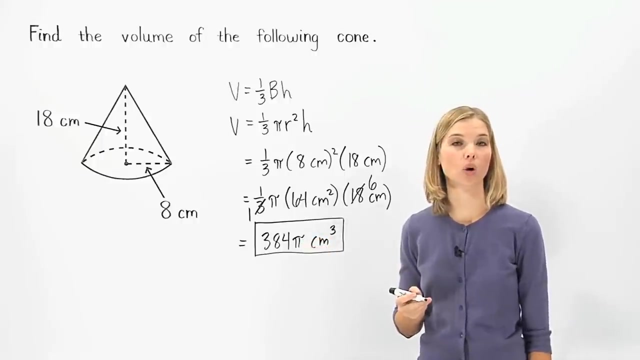 times 6 centimeters, which simplifies to 384 pi centimeters cubed. So one way to write the volume of the given cone is 384 pi cubic centimeters. Next, remember that pi is approximately equal to 3.14..